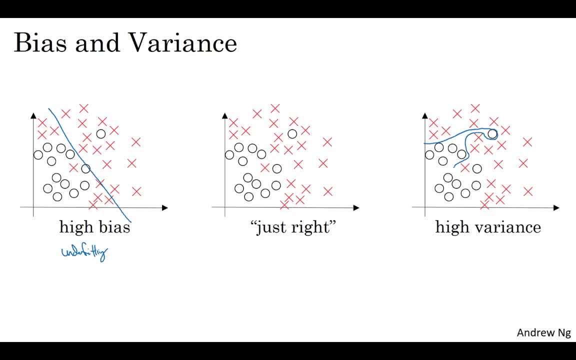 a neural network with a lot of hidden units. maybe you can fit the data perfectly, but that doesn't look like a great fit either. So this is a classifier with high variance and this is um overfitting the data, And there might be. 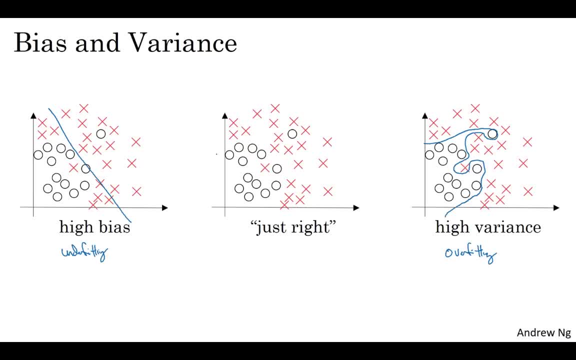 some classifier in between with a medium level of complexity that you know, maybe fits a curve like that, that looks like a much more reasonable fit to the data, and so that's the we call that. you know, just right right, somewhere in between. 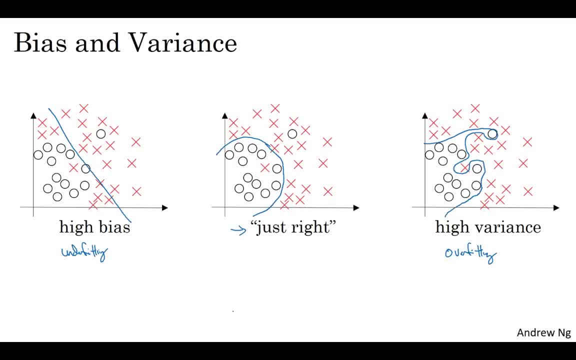 So in a 2D example like this, with just two features, x1 and x2, you can plot the data and visualize bias and variance In high dimensional problems. um, you can't plot the data and visualize the decision boundary. 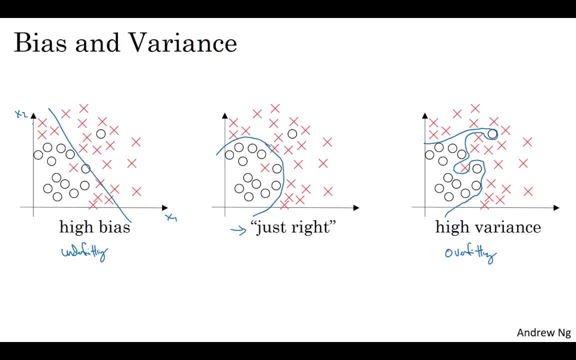 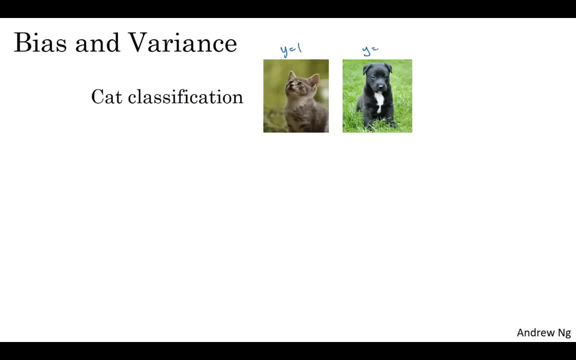 Instead, there are a couple of different metrics that we'll look at to try to understand bias and variance. So, considering our example of cat picture classification, where that's a positive example and that's a negative example, the two key numbers to look at to understand bias and 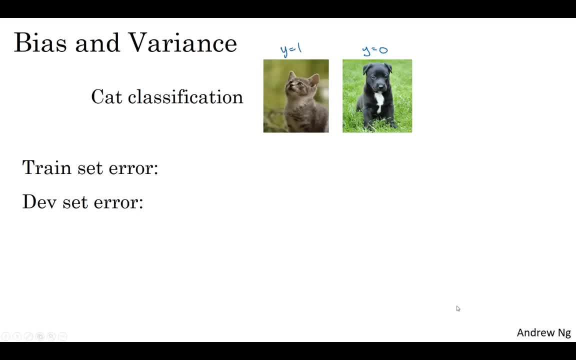 variance will be the training set error and the def set or the development set error. So, for the sake of argument, let's say that, um, you know, recognizing cats and pictures is something that people can do nearly perfectly right. And so let's say your training set error is um 1%. 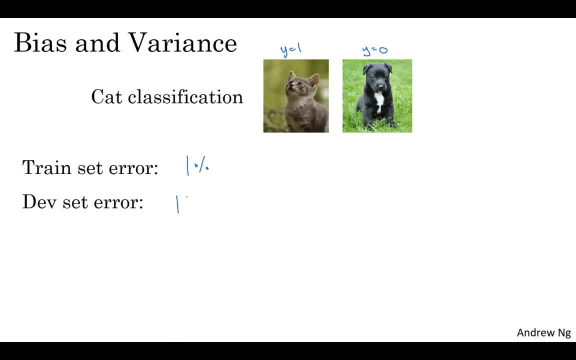 and your def set error is uh. for the sake of argument let's say it's 11%. So in this example, you're doing very well on the training set, but you're doing um relatively poorly on the development set. 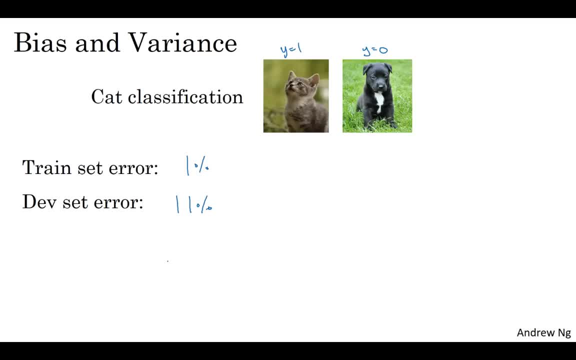 So this looks like you might have overfit the training set that somehow you're not generalizing well to this whole dark cross-validation set or the development set, And so if you have an example like this, we will say this has high variance. 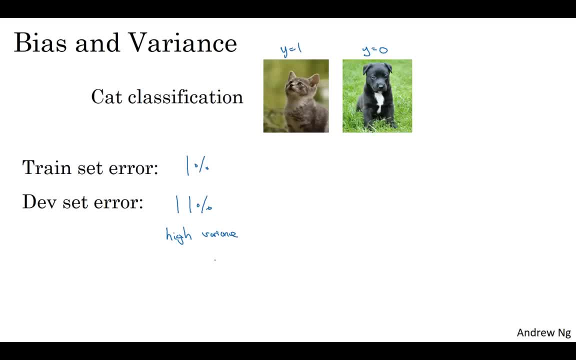 So by looking at the training set error and the development set error, you know you would be able to render a diagnosis of your algorithm having high variance. Now let's say that you measure your training set and your def set error and um you get a different result. 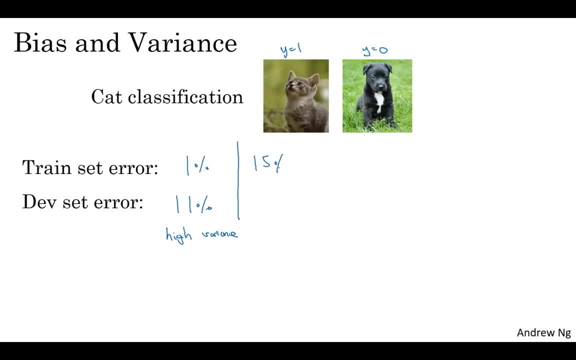 Let's say that your training set error is 15%. I'm writing your training set error in the top row and your def set error is 16%. In this case, assuming that humans um achieve, you know, roughly 0% error. 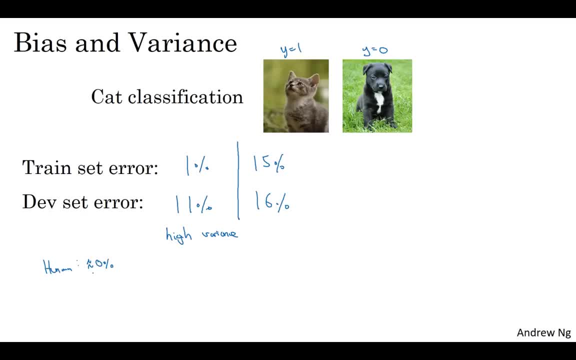 that humans can look at these pictures and just tell if it's a cat or not, then it looks like the algorithm is not even doing very well on the training set. So if it's not even fitting the training data as seen that well, then this is underfitting the data. 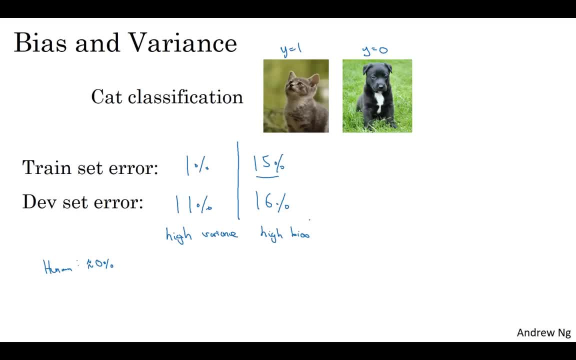 and so this algorithm has high bias. But in contrast, this is actually generalizing at a reasonable level to the def set, Whereas performance of def set is only 1% worse than performance on the training set. So this algorithm has a problem of high bias because um 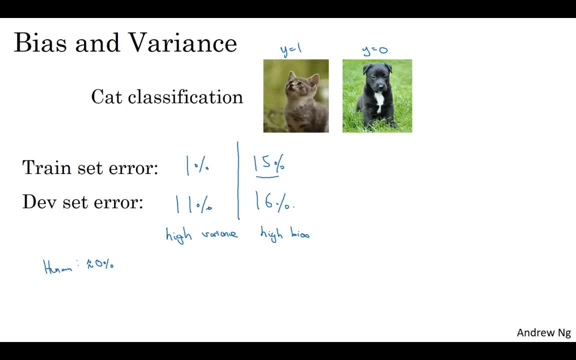 well, it's not even training, it's not even fitting the training set. well, This is similar to the leftmost plot we had on the previous slide. Now here's another example. Let's say that you have 15% training set error. 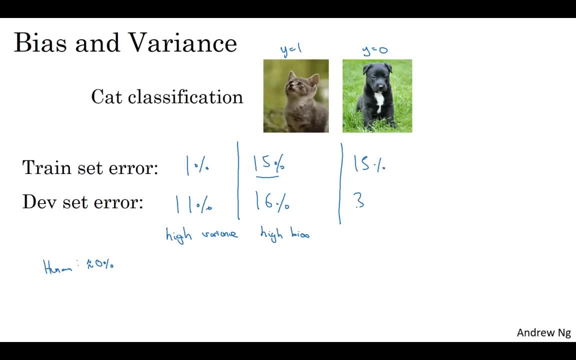 so that's pretty high bias. But when you evaluate on a def set, it does even worse. Maybe it does, you know, 30% In this case. I would diagnose this algorithm as having high bias because it's not doing that well on the training set. 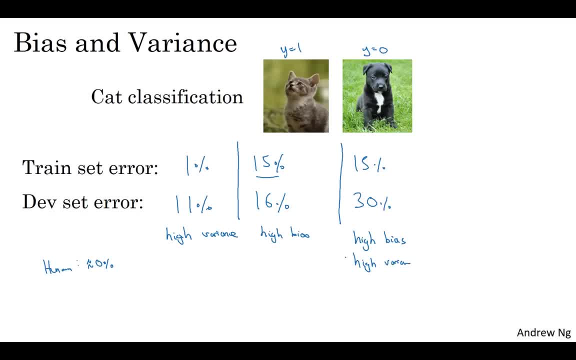 and high variance. So this is, you know, really the worst of both. Um. and one last example: if you have, you know, 0.5 training set error and 1% def set error, then well, maybe your users are quite happy that you have. 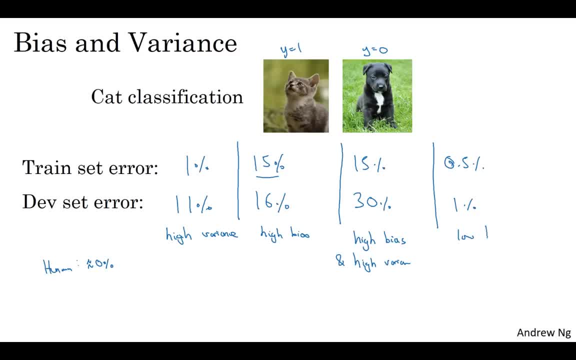 uh, a classifier with only 1% error, then this would have, you know, low bias and low variance. One subtlety that I'll just briefly mention, but we'll leave to a later video to discuss in detail, is that this analysis is predicated on the assumption that 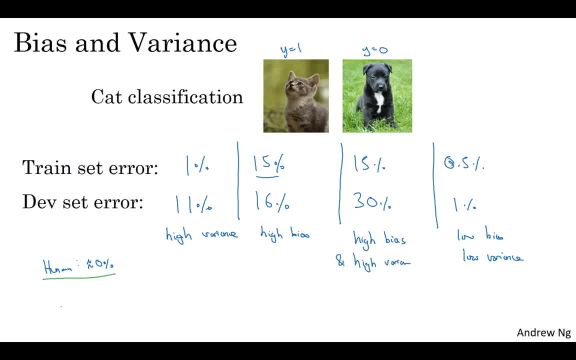 human level performance: yes, nearly 0% error. Or, more generally, that the optimal error, sometimes called Bayes error for the. so the Bayesian optimal error is nearly 0%. I don't want to go into detail on this in this particular video. 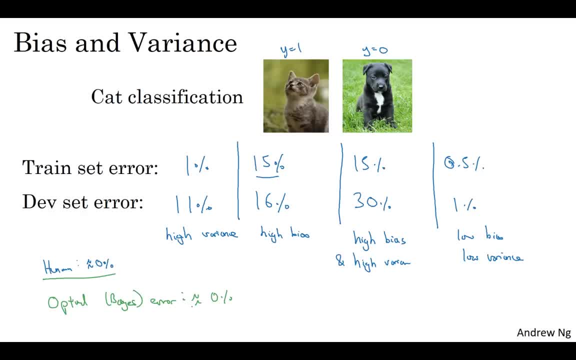 but it turns out that if the optimal error or the Bayes error were much higher- say it were 15%- then if you look at this classifier, um, 15% is actually perfectly reasonable for a training set and you wouldn't say that's high bias. 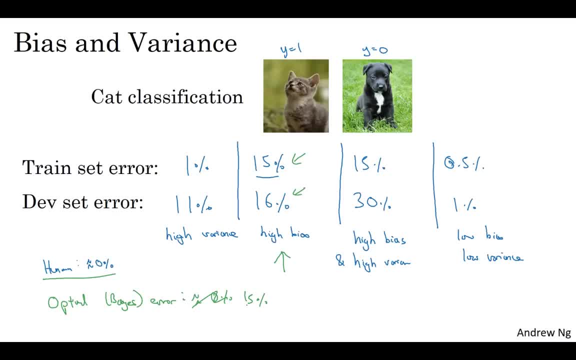 And it wants a pretty low variance. So the case of how to analyze bias and variance when no classifier can do very well, for example, if you have, um, really blurry images, so that you know even a human or just no system could possibly do very well. 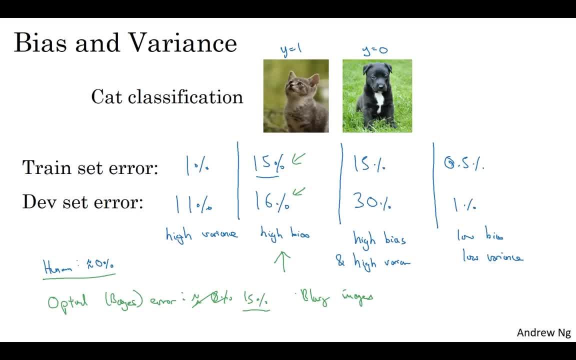 then maybe Bayes error is much higher, and then there's some details of how this analysis would change. But leaving aside this subtlety for now, the takeaway is that by looking at your training set error you can get a sense of how well you're fitting at least the training data. 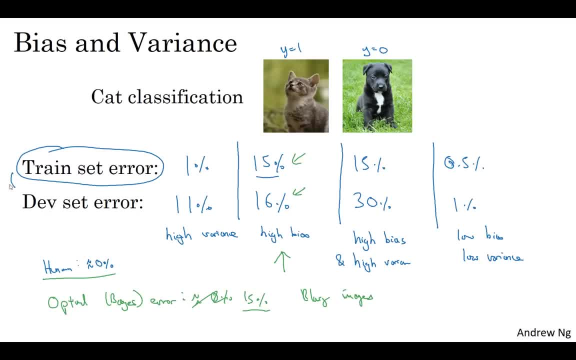 and so that tells you if you have a bias problem. And then looking at how much higher your error goes when you go from the training set to the depth set, that should give you a sense of how bad is the variance problem. So you're doing a good job generalizing from the training set to the depth set. 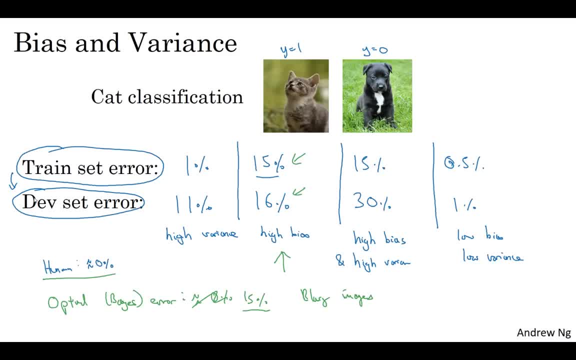 That gives you a sense of your variance. All this is under the assumption that the Bayes error is quite small and that your training and your depth sets are drawn from the same distribution. If, if those assumptions are violated- uh, there's a more sophisticated analysis you could do. 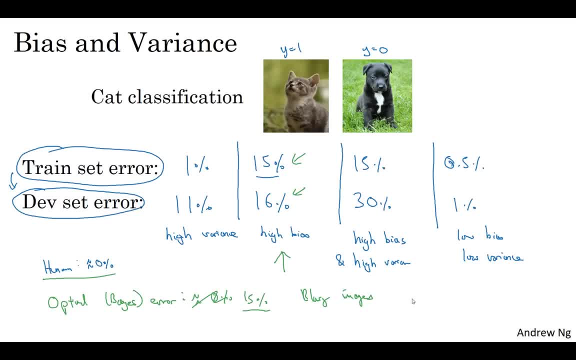 which we'll talk about in the later video. Now, on the previous slide you saw what high bias, high variance looks like and I guess you had a sense of what a good classifier looks like. What does high bias and high variance looks like? 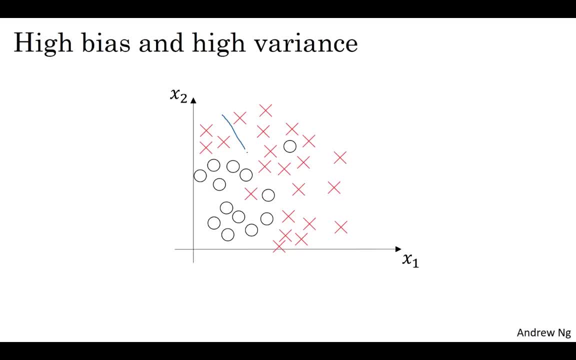 It's kind of the worst of both worlds. So you remember we said that a classifier like this, a linear classifier, has high bias because it under fits the data. So this would be a classifier that is mostly linear and therefore under fits the data. 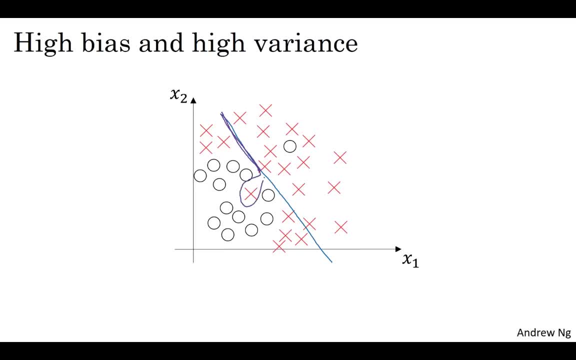 We're drawing this in purple, But if somehow your classifier does some weird things, then it's actually overfitting parts of the data as well. So the classifier that I drew in purple has both high bias and high variance. Right, that's high bias because by being a mostly linear classifier,